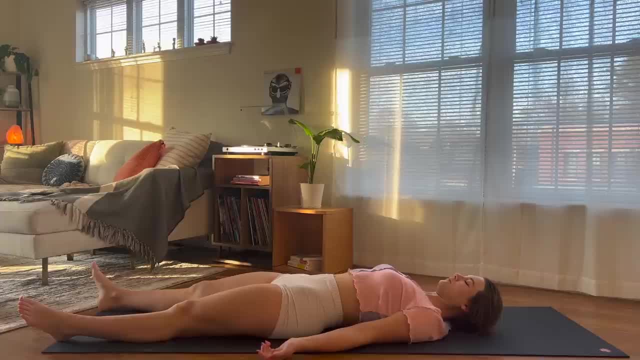 to settle into your space. As I mentioned, this is a low back focused flow, Some twists and hip openers throughout, And this quick sequence will help bring relief to your low back and spine. Place your left palm on your heart, right palm on your belly And notice the rise and fall of your chest. 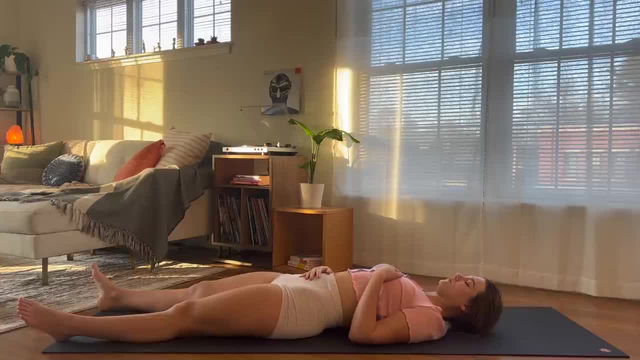 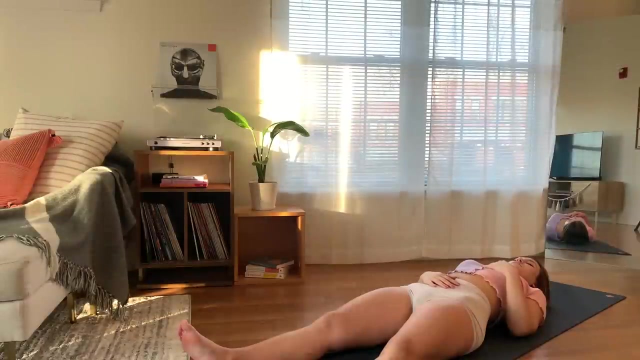 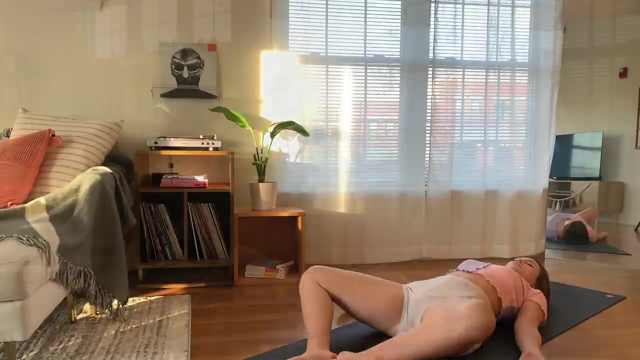 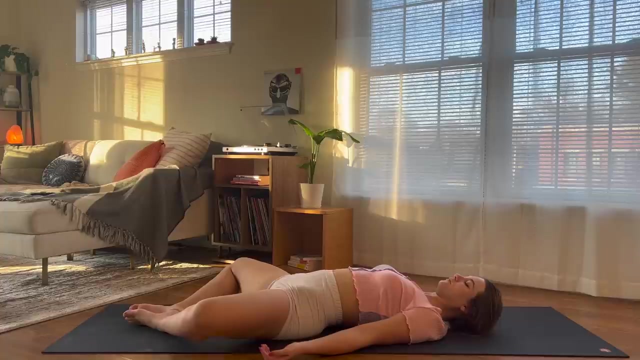 and belly with each inhale and exhale. Release your arms long by your side, Bend through your knees, Bring the soles of your feet together for supta baddha, konasana, or butterfly, pose within your legs Here for just a moment. Breathe through your legs And release your arms long by your side. 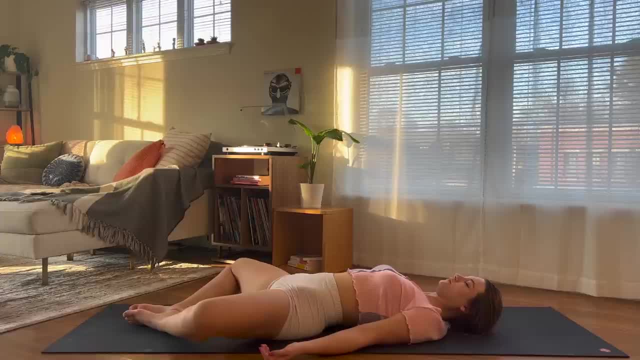 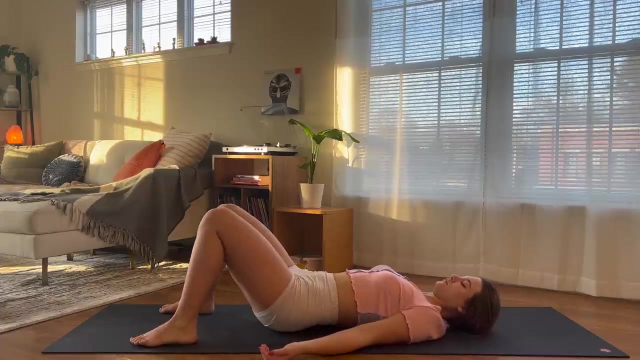 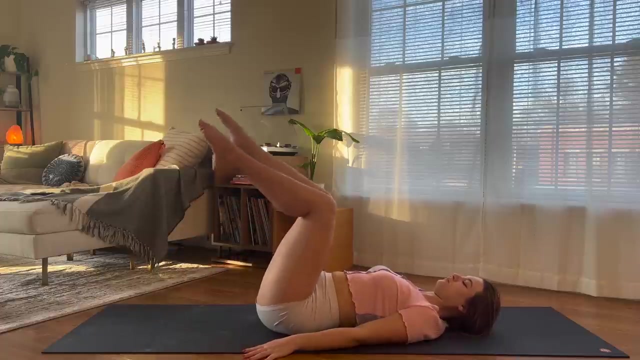 When you're ready, bring your knees close together and plant your feet on the mat, Preparing for supine twist. lift your feet off the mat. Stack those knees on top of your hips. Scooch your hips over to the right side of your mat. Have your knees on top of your 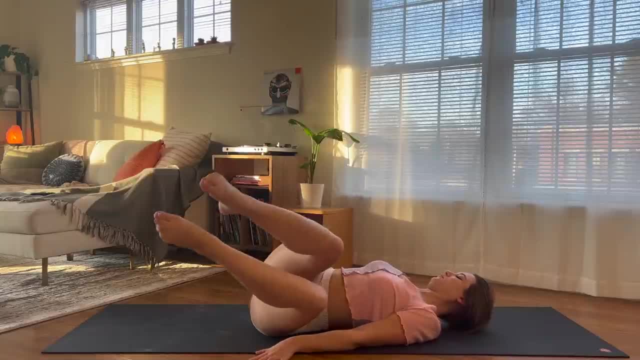 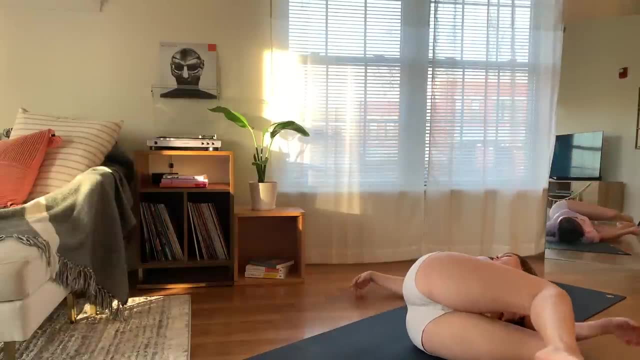 hips And lift your feet off the mat, Bring your arms out at a T And let your legs fall over to the left side of your mat, Coming into that supine twist. Your legs can be stacked on top of one another or they can. 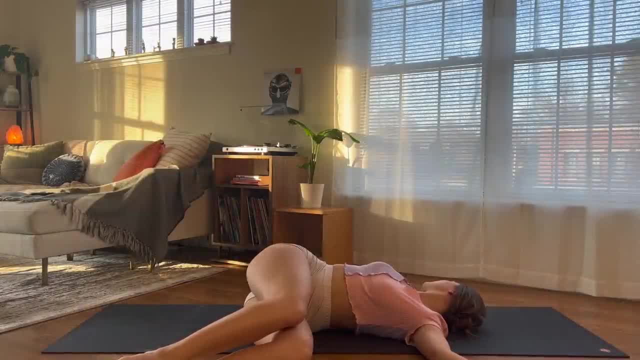 be in a staggered position. Whatever feels good, Gaze is to the right. Bring your awareness to your spine And feel into this twist. Bring your head down, Using the knee, bringing the bud of your besten, Coming into that supine twist. Yup. 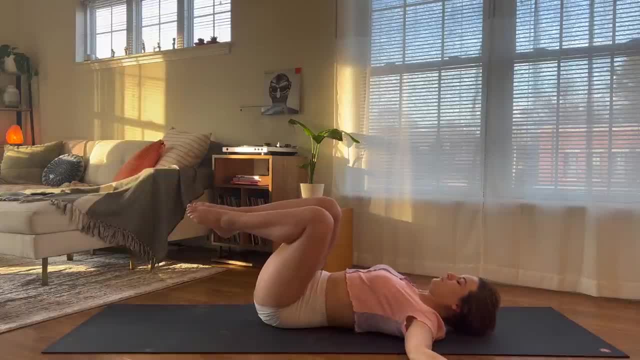 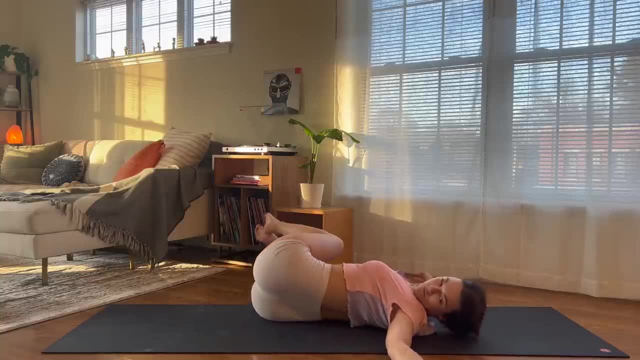 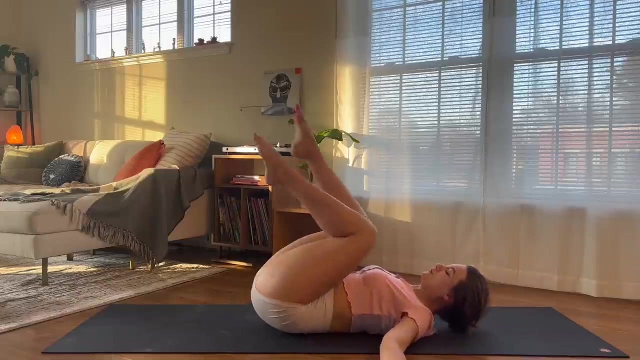 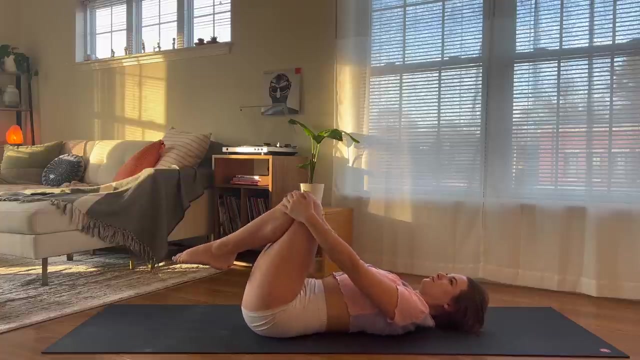 Decide not to bend your arms or lower your arms. Those of you who are ready, this is your second 50 reps of supine twist. get your Come back through center, bring those knees close to your chest, hands on your shins or 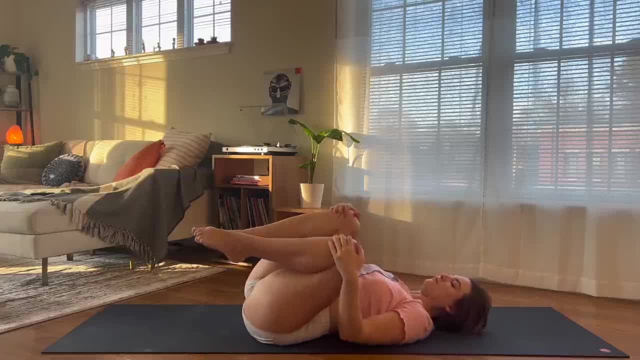 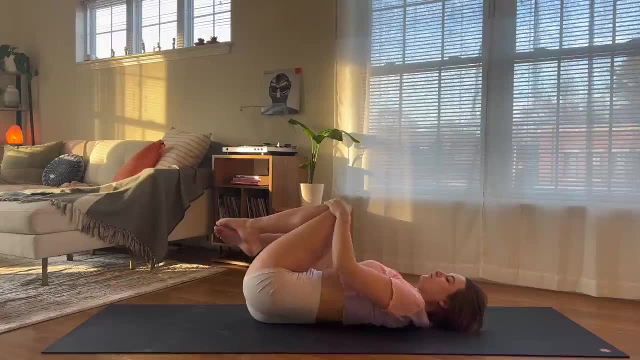 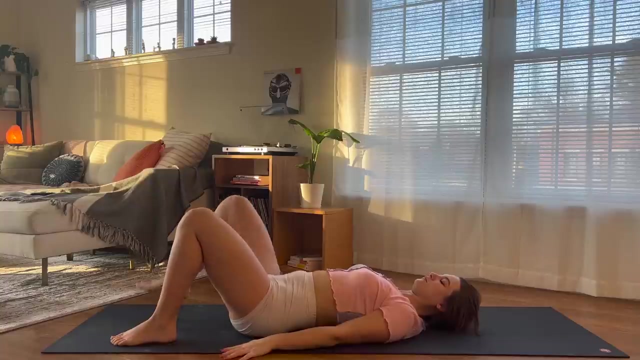 knees. in a tiny ball You can take some tiny circles for your low back, going in one direction a couple of times before switching to the opposite. Now plant your feet on the mat. Begin to cross your right ankle on top of your left thigh. option to stay here for a. 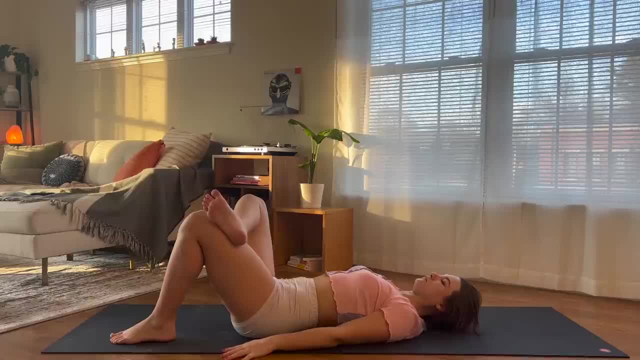 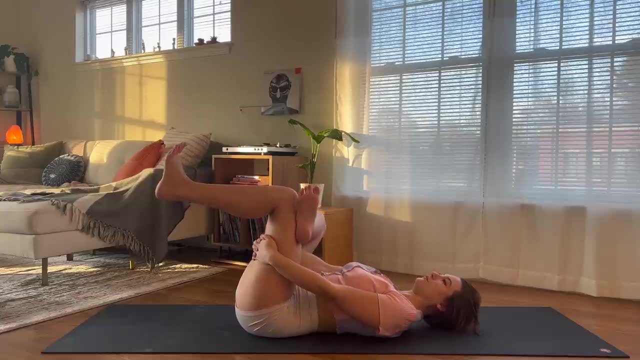 gentle hip opener. or you can go deeper by lifting the left foot off the mat. interlace your hands behind your left thigh and pull that leg closer to you. Your feet should both be flexed, so toes pointed towards the sky and ground down through your. 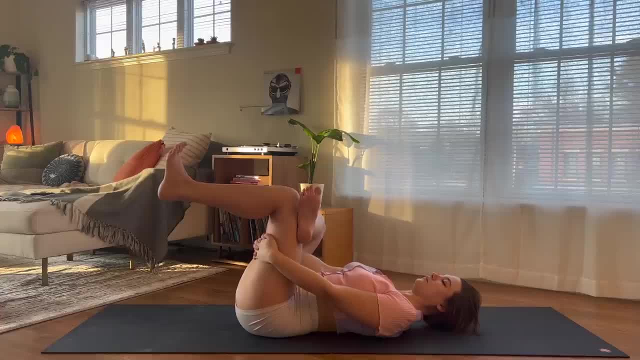 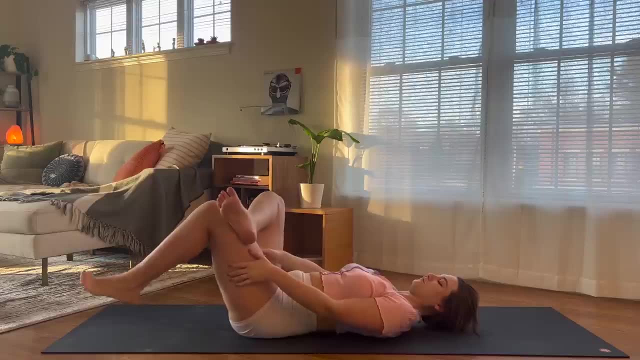 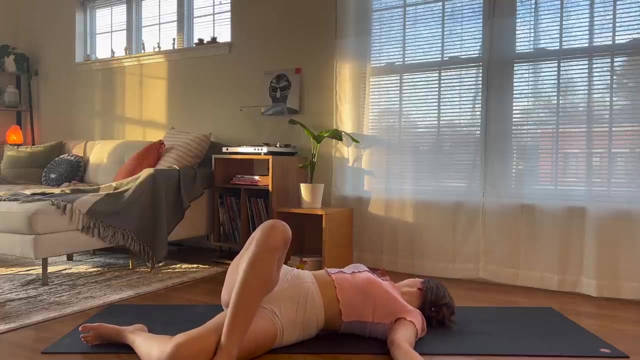 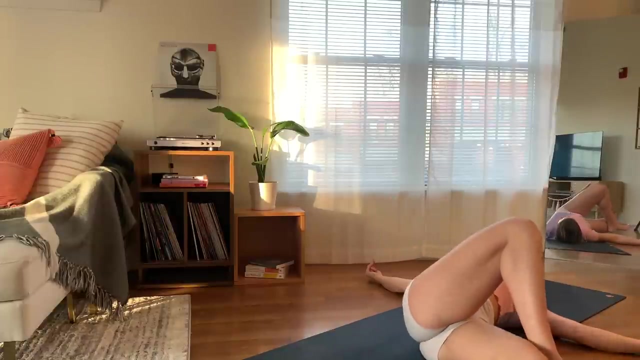 low spine. Take a deep inhale and as you exhale, slowly lower the left foot down to the mat. Keep that right ankle crossed on top of your left thigh and just let your legs follow out and make sure you don't fall over to the left side of your mat. 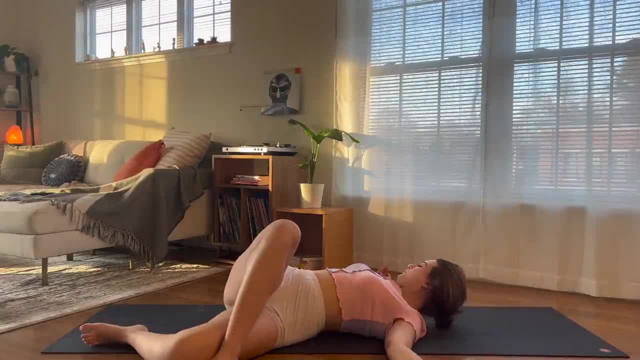 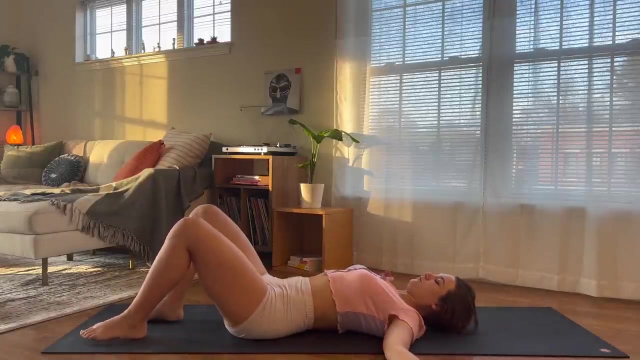 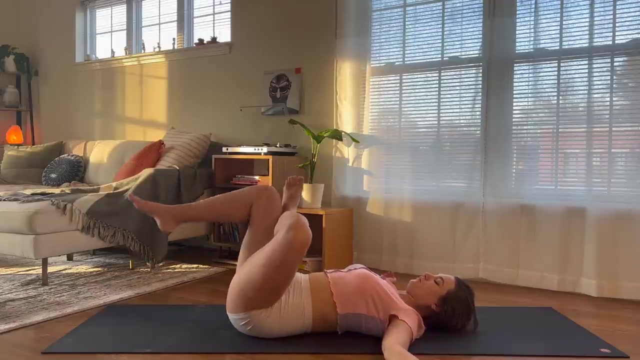 Come into this gentle twist. That right foot is planted on the ground, gaze can be toward the right. Come back through center when you're ready and release the legs, Switching it out. Cross that left ankle on top of your right thigh. 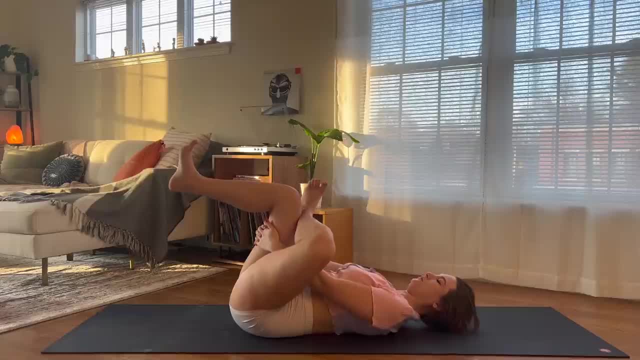 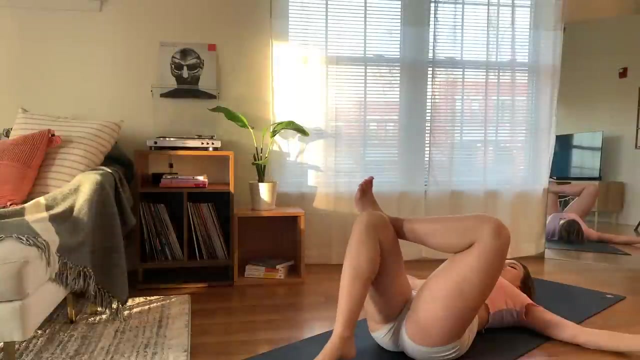 figure four pose and either stay here or go to the deeper stretch. lift the right foot off the mat, interlace your hands and again ground down through your low spine, deep inhale and exhale. plant the right foot and come to that gentle twist on this side. 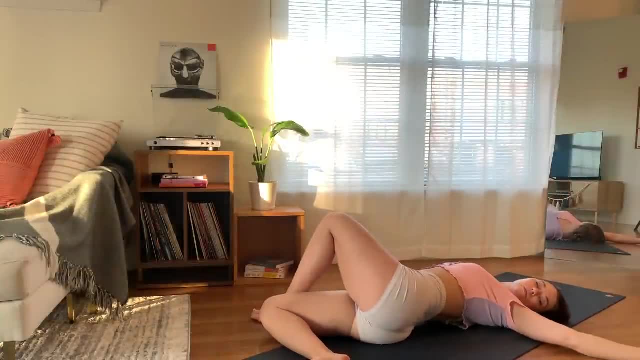 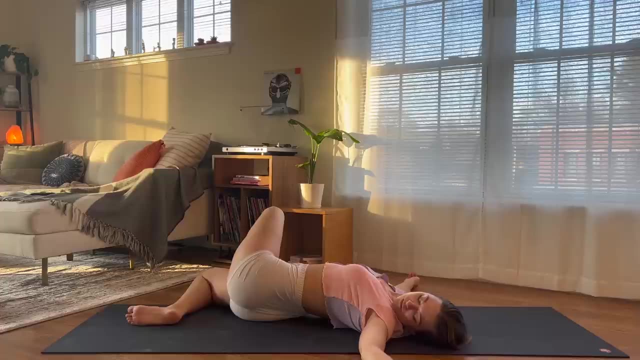 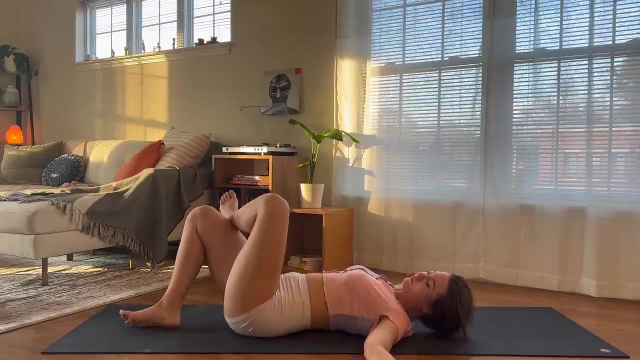 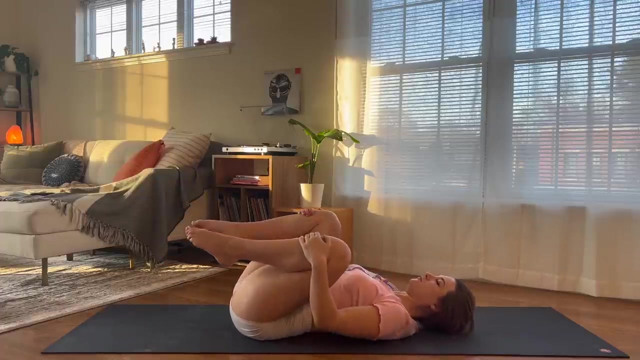 letting those legs fall over to the right, left foot plants down, come back through center and plant both your feet on the mat. coming in into ananda, balasana or happy baby, so bring those knees close to your chest and body. now widen out your legs and thighs about. 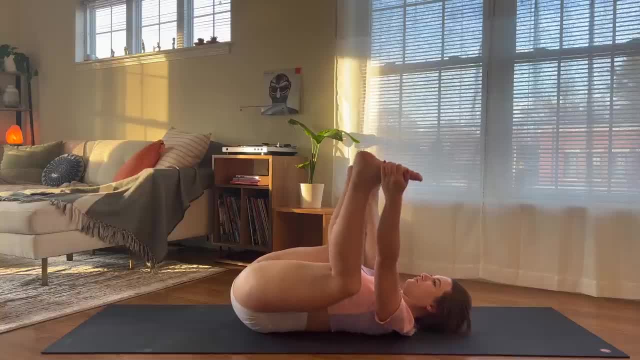 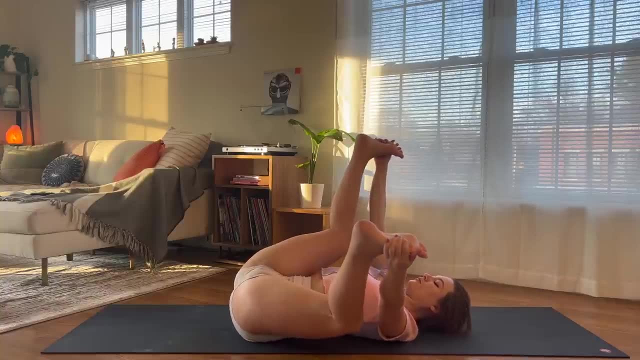 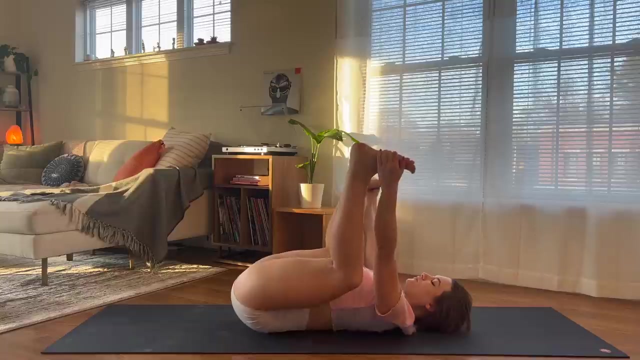 the width of your torso, bring those knees towards your armpits, ground down through your low spine and take a hold of your feet, toes or ankles. rock side to side, feel the breath in and out, make those hips contoured, speak your breath gently, trunk the ambundance to your chest. 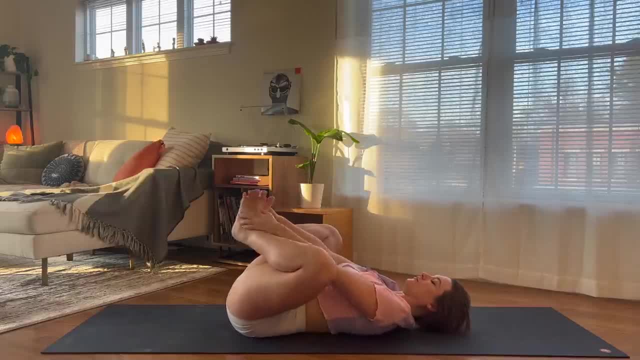 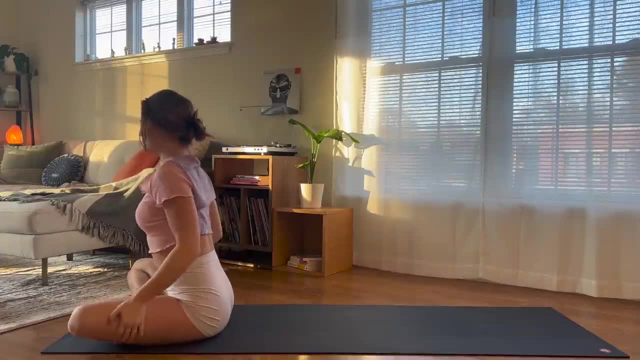 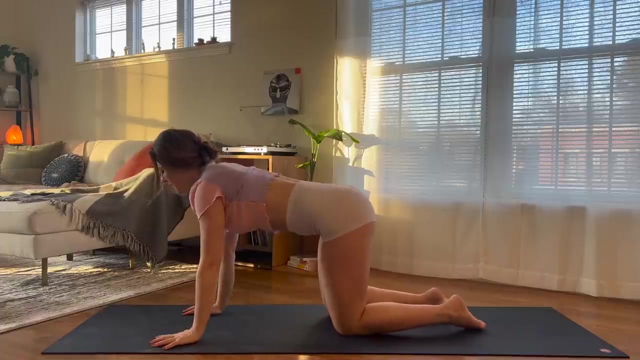 bring those feet to the ground beneath you, engage your core as you ground down using the heels through your back, begin to gently release out of your happy baby into a tiny ball, then rock yourself forward and make your way into a tabletop position. once you are in position for this type of move, i will go ahead and ocho phase isords in the anal. 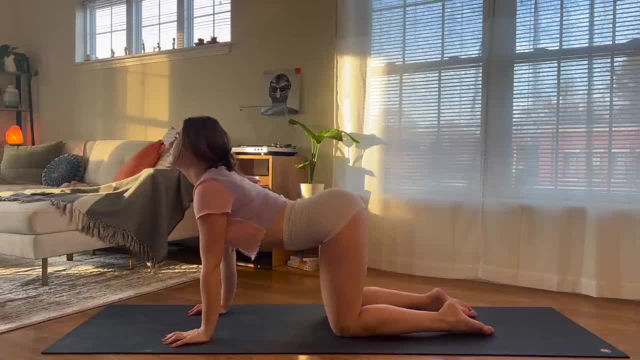 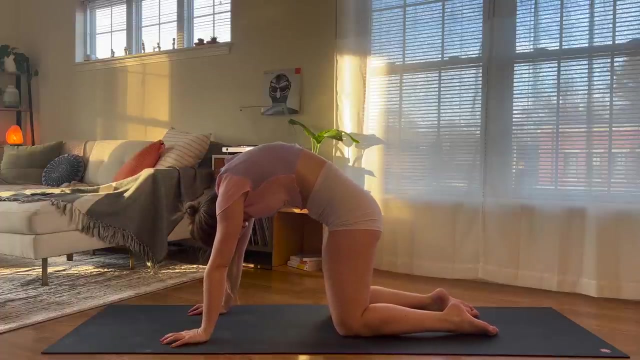 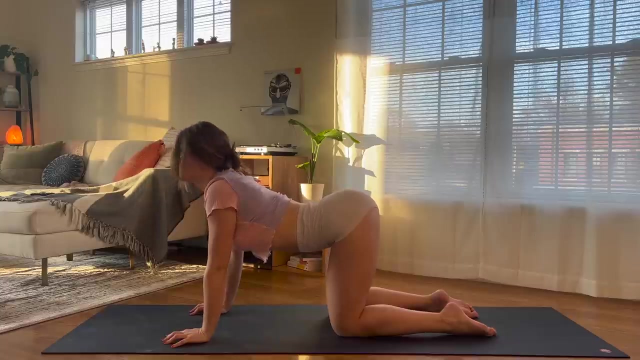 in table. go right into your cow and cat pose so as you inhale you'll drop your belly, lift your gaze, shine through your heart. cow pose: exhale cat round through your upper spine, press the ground away from you. inhale, drop the belly, lift your gaze, exhale cat around your spine and go ahead and take a few more rounds of your. 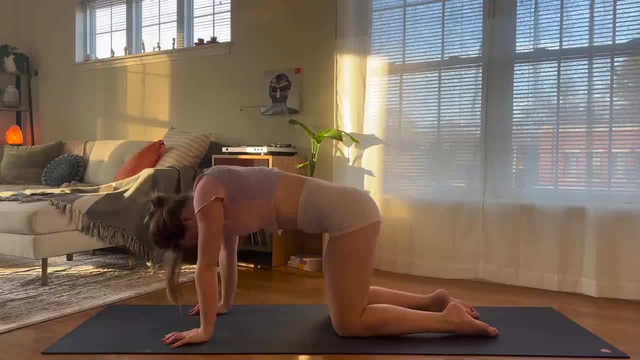 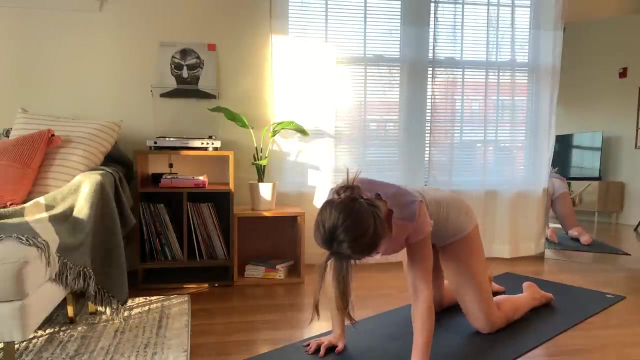 cow and cat paired with your breath. if you'd like to add in some spinal rolls, feel free to do so and while you're here, I encourage you to really accentuate these movements, really feel ensuring that you're breathingely purely to your feeling. though, show some self-care. C to the left and make sure that you sit магазin. 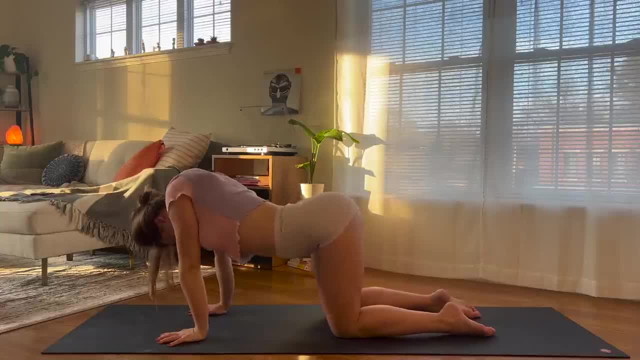 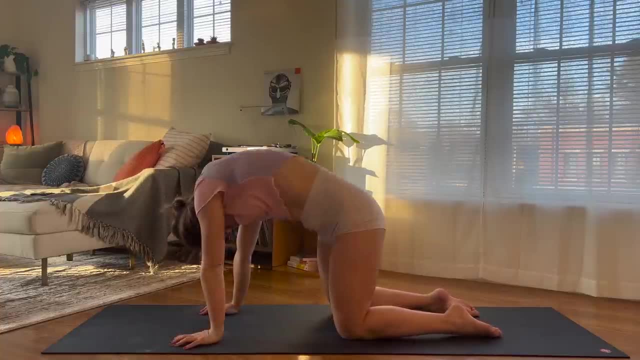 不要 putry the eyes forward until you become a man. esta la preson todo rosa nueva. your body and spine. give yourself a chance to just move in a way that feels really good for you. come back to a neutral spine in your tabletop, ground down through your left. 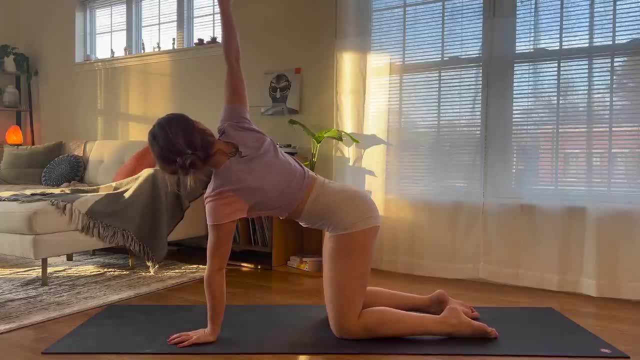 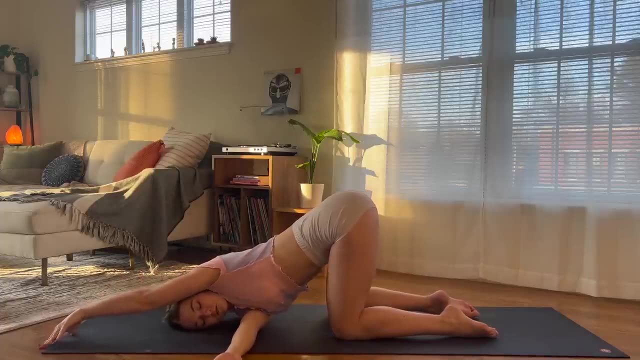 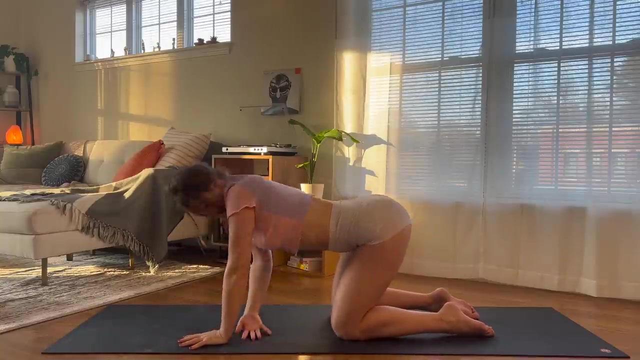 palm. inhale. right arm reaches all the way up and exhale thread the needle. bring that right arm towards the left side of your mat, right temple towards the mat. left palm is reaching towards the top of your space. nice twist here. bring that left palm back down underneath your shoulder and push. 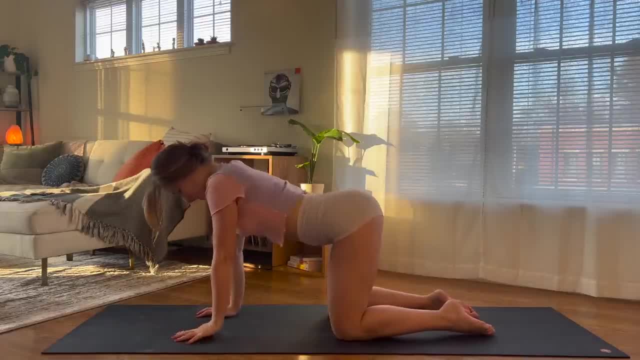 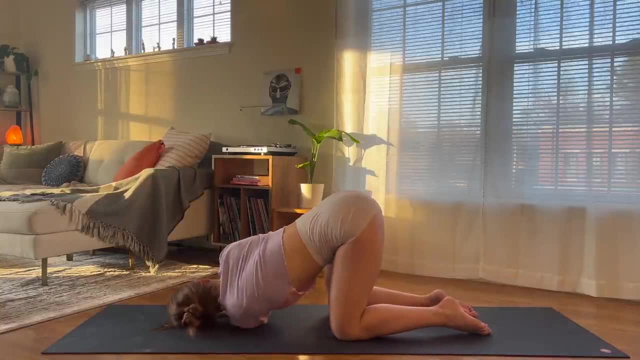 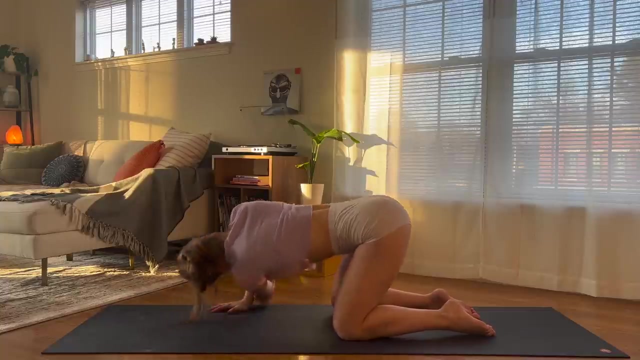 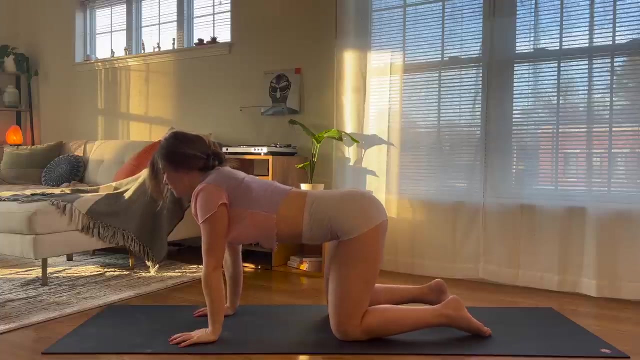 yourself up out of this pose back into your tabletop, switching sides. ground down through the right palm. left arm reaches up and as you exhale, thread the needle reaching that right palm towards the top of your mat. gently begin to release out of this pose. come back to your tabletop as you inhale. 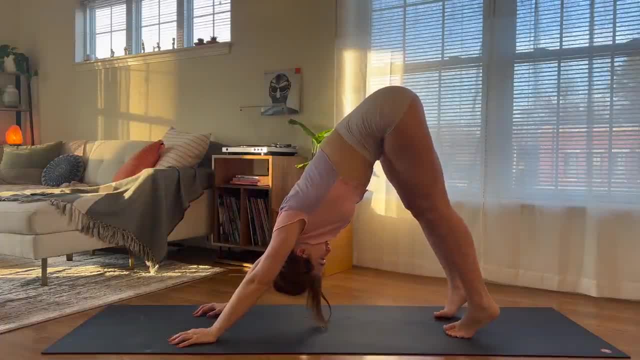 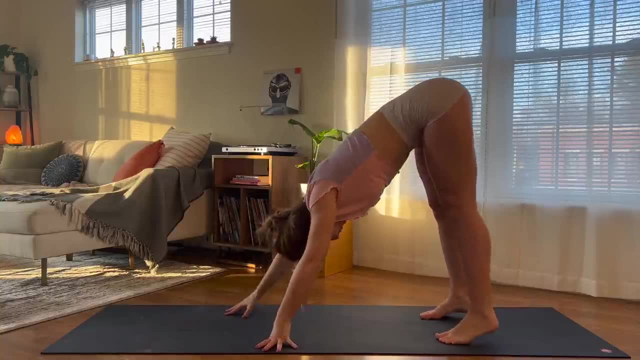 flip your toes- exhale. lift your hips. straighten out those legs downward, dog. exhale, lift your hips. straighten out those legs downward, dog. exhale. lift your hips. straighten out those legs downward, dog. now begin to walk those palms towards your feet, at the back of your space, into. 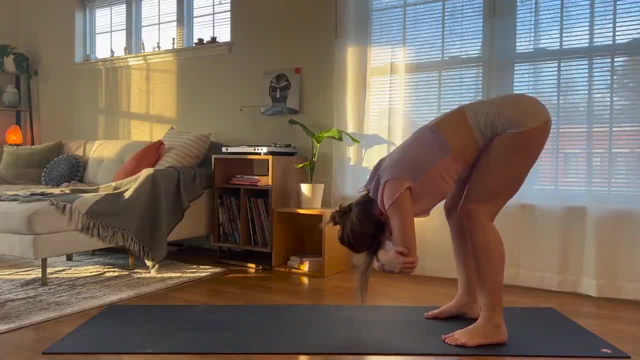 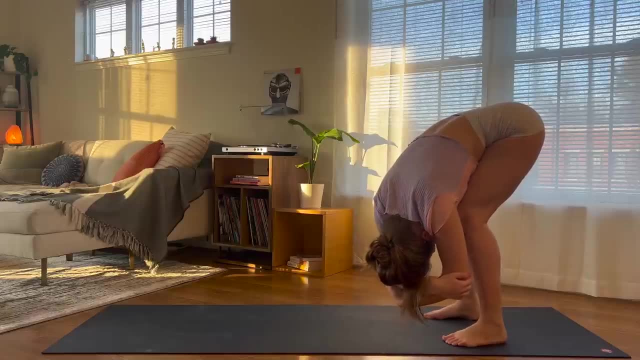 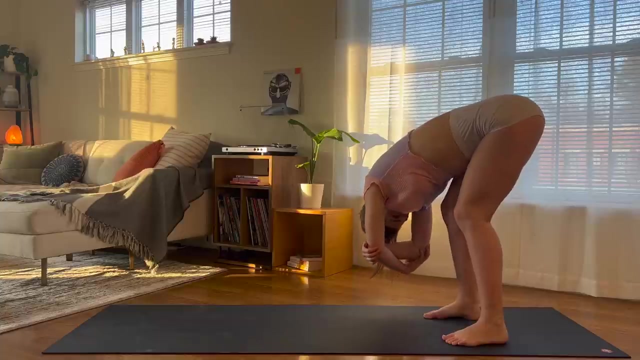 a forward fold. widen out your stance a little bit and come into ragdoll pose. so bend through your knees so much that your chest is falling on top of your thighs. take a hold of opposite elbows and sways side-to-side. ground down through your feet, your feet. let your torso fall heavy. now release your hands down to the mat, walk. 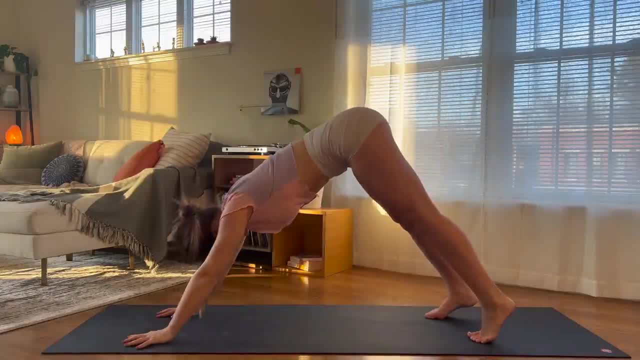 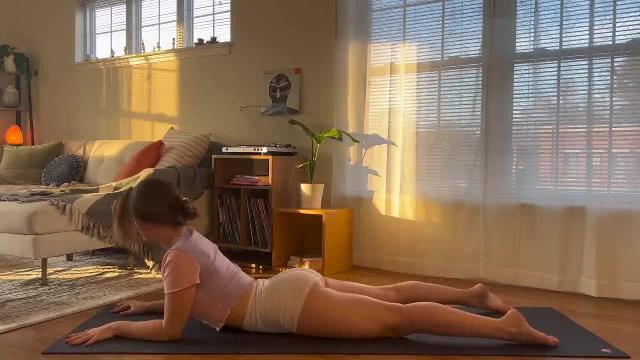 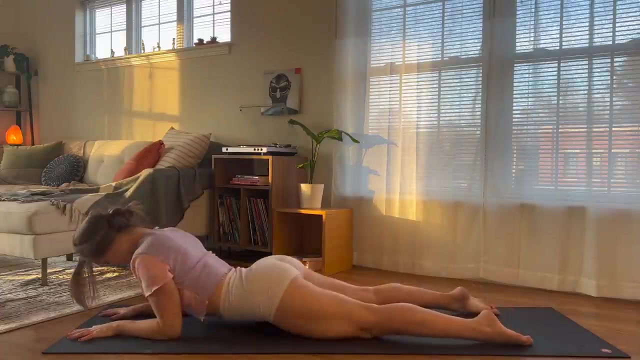 yourself out into a plank position and lower all the way down to your belly. prop yourself up onto your forearms. make sure your elbows are underneath your shoulders. arms are in a parallel position, round down through your hip bones. lift through your chest, press into your forearms deep inhale and exhale. 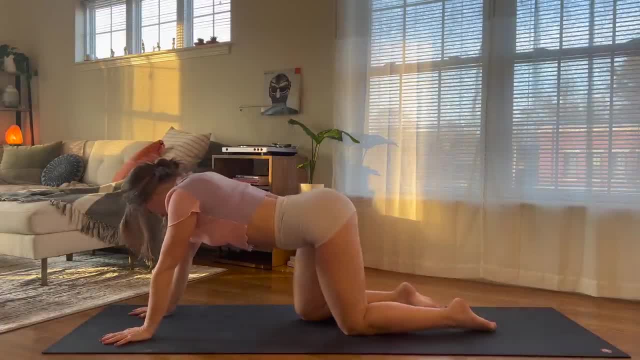 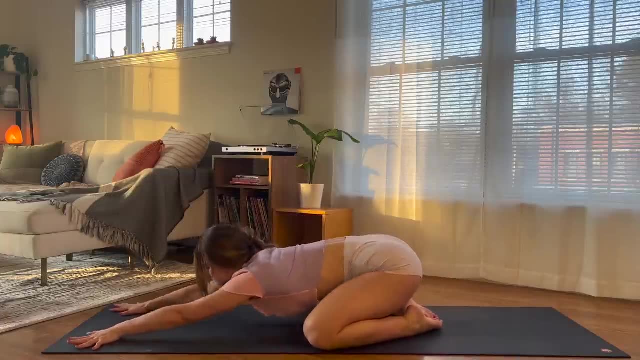 begin to push yourself up and back into a tabletop position. then come to a child's pose, widen out your knees about the width of your feet and bring your arms down to the mat, walk yourself out into a plank position and lower all the way down to your belly. 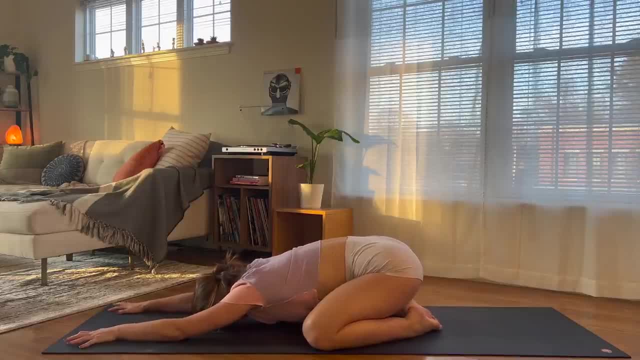 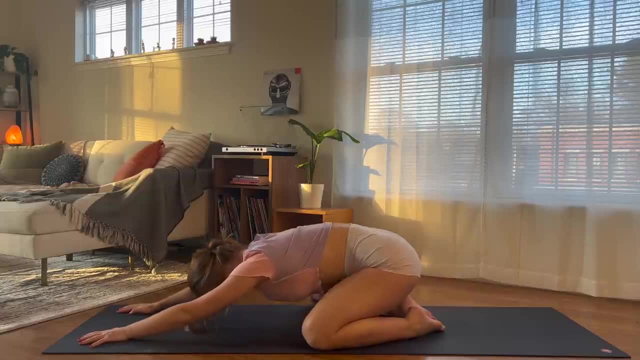 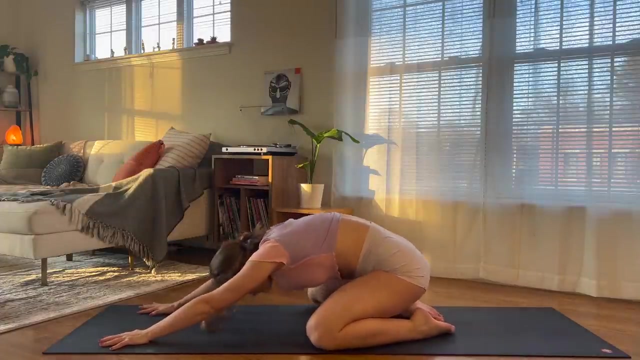 mat big toes come to touch, sink those hips to your heels and reach those palms forward here briefly, before you push yourself back up into a tabletop and then sink yourself back into your child's pose. doing this back and forth motion between your table and child's pose a few times again really accentuate these. 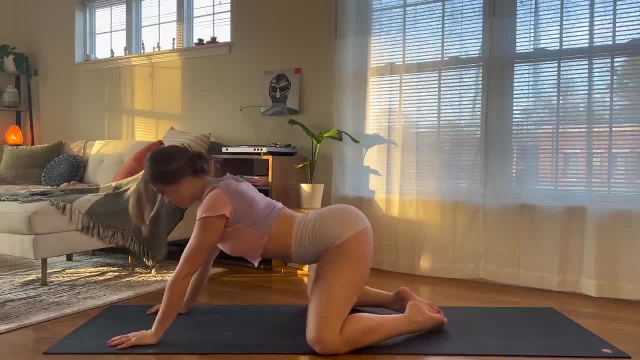 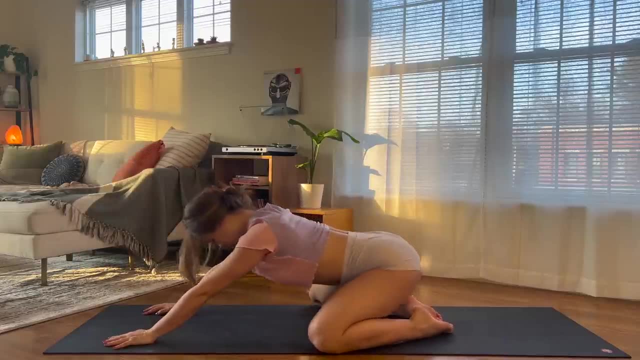 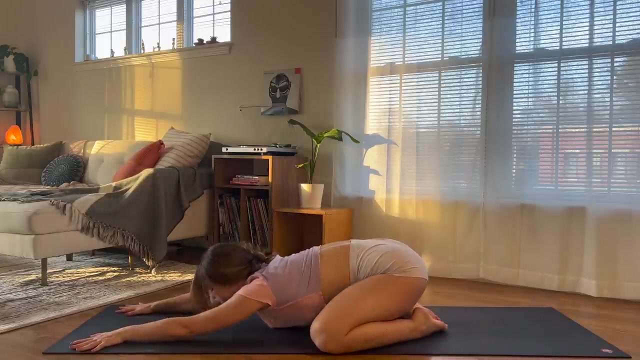 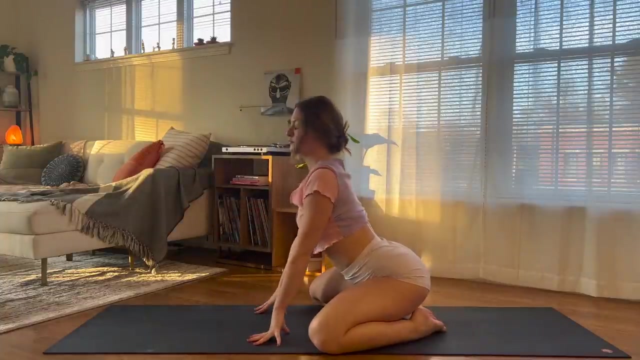 movements feel into your body and, after you've taken a few rounds, sink back into your child's pose, reaching through your fingertips towards the top of your mat, lengthen through your spine in your child's pose and, when you're ready, gently push yourself up out of your child's pose and make your way into a 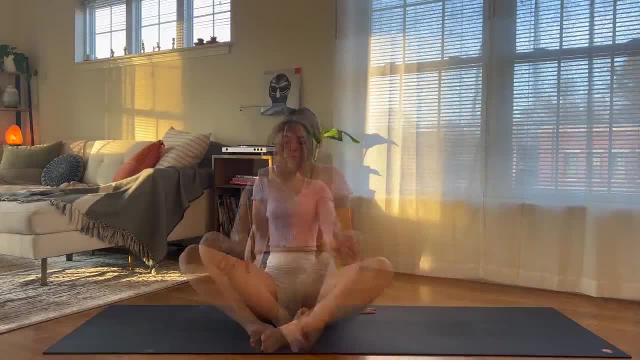 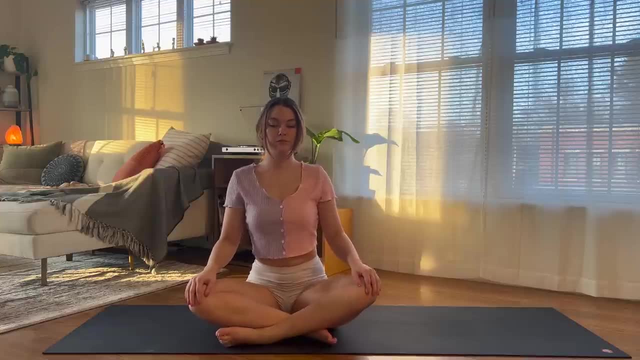 comfortable seat. legs are crossed, ground down through your tailbone. lift through your chest, bring your left palm to your heart, right palm to your belly. eyes are closed, inhale and exhale on your next. inhale gently, open your eyes. reach those arms high above your head, round down through your tailbone and exhale palms together at